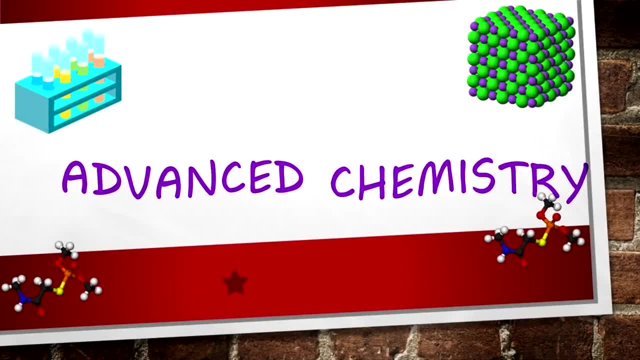 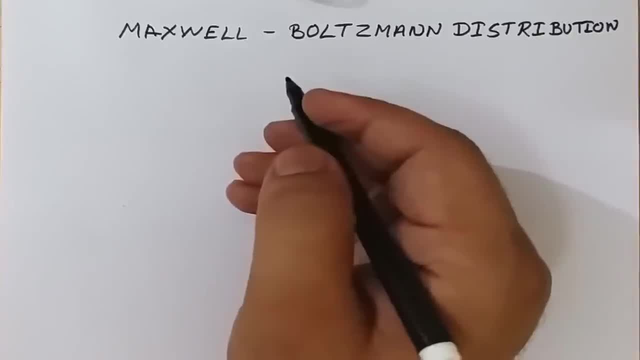 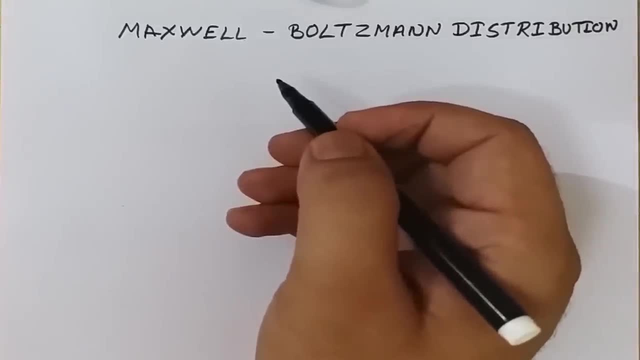 Hey friends, welcome. today we are going to discuss a Maxwell Boltzmann distribution and in this distribution we are going to see that how large number of particles are most probably distributed, and for that we will consider that we will take a system which contains n number of identical. 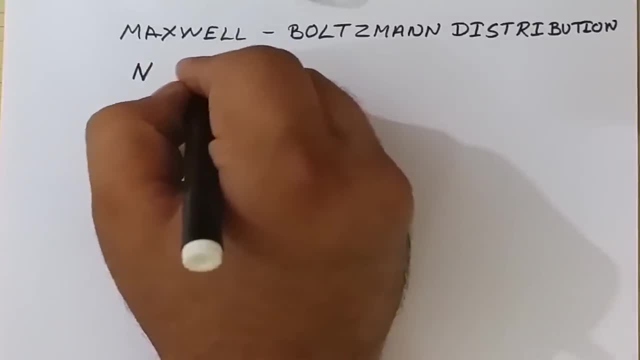 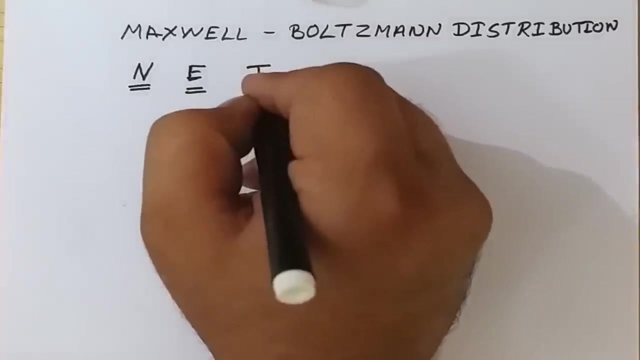 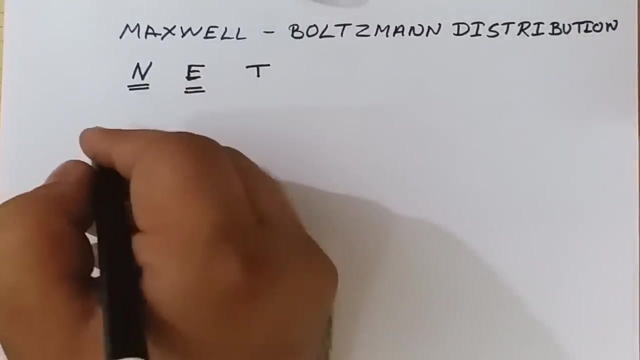 particles with constant energy, e, So our, in this system, the total number of particles as well as the total energy of the system remains constant and at constant temperature. So at constant temperature. now, this or this system has several constraints and there are several assumptions made in deriving Boltzmann distribution law. 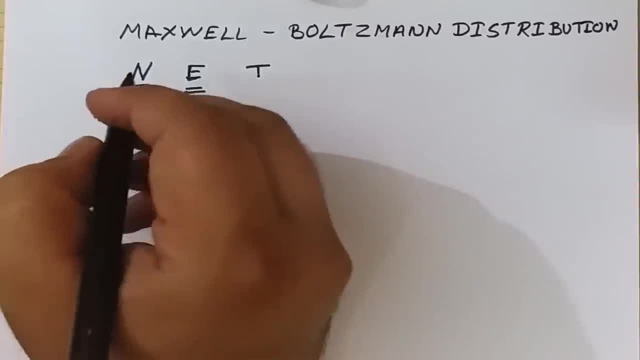 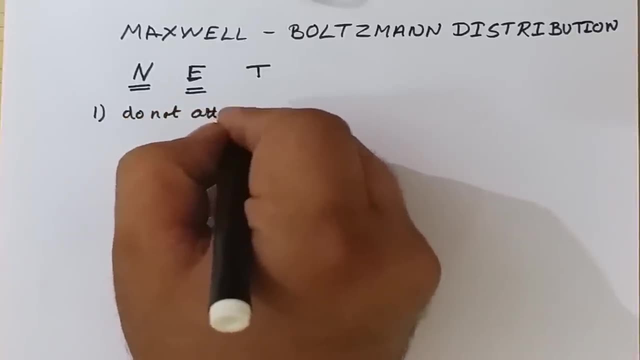 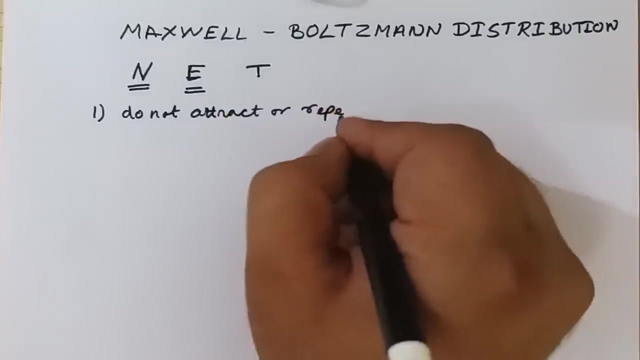 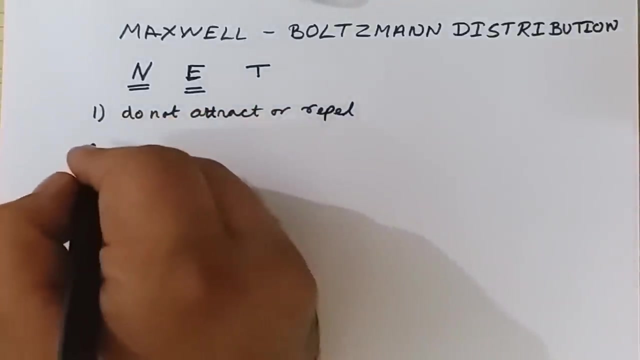 So the first assumption made is that the particles, they do not attract or repel each other. so they do not attract or they repel each other means there is no attractive or repulsive force between each other. so they are, they are not affected by the inter nuclear interactions. The second assumption: 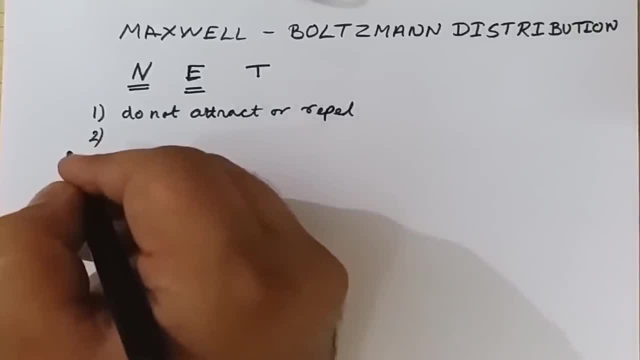 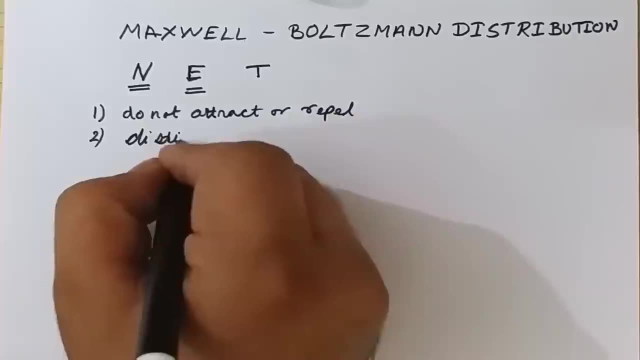 made is that each particle is distinguishable between the two particles. The second assumption made is that the particles, they do not attract or repel each other. so they do not attract or repel each other. so the second part is: each particle is distinguishable. so distinguishable, that means we can identify. 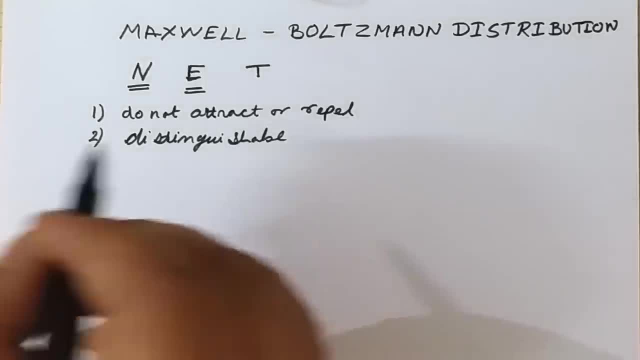 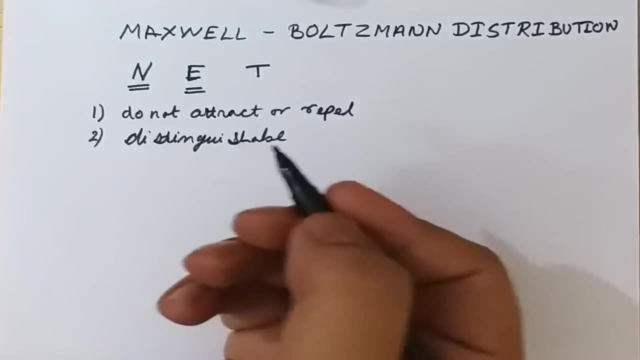 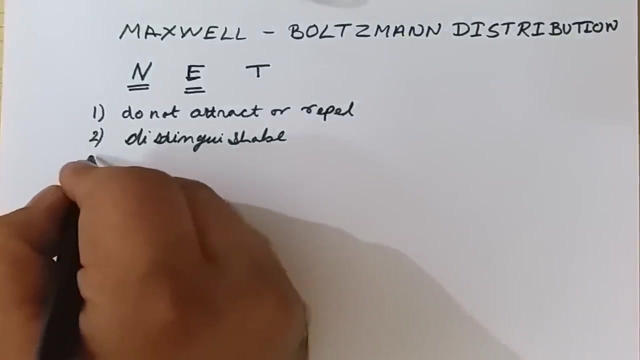 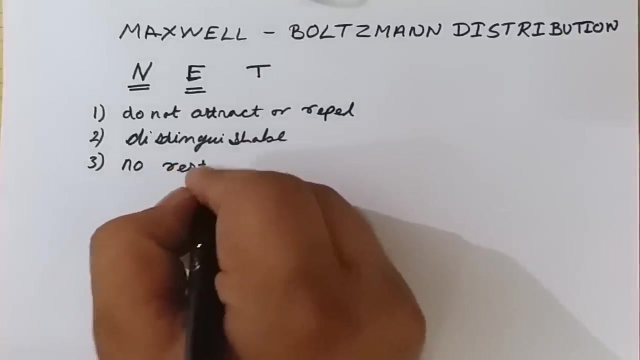 particle, where a particular particle is laying in our different energy levels, like in a classroom. we have identified or distinguishable students, so we may how we are easily able to identify the particles are distinguishable. the third is that the no restriction is being imposed on arrangement of various energy levels to the particle, so there is no restriction on the arrangements of the 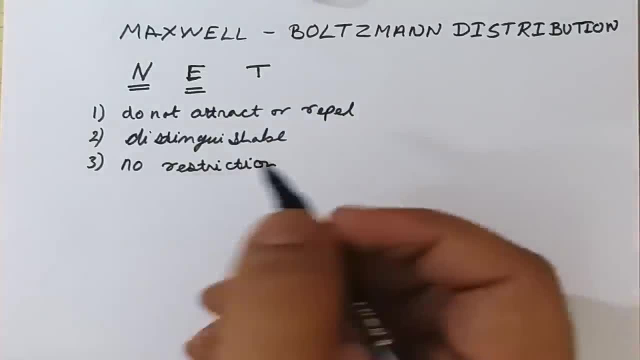 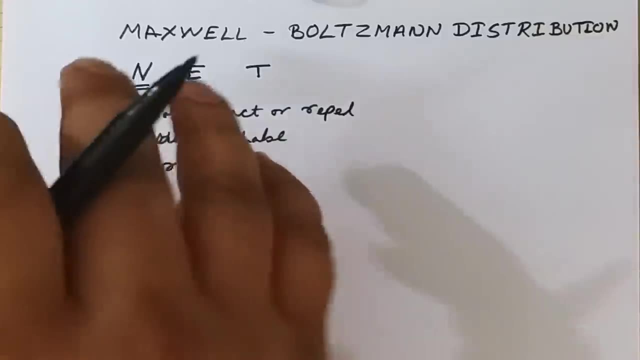 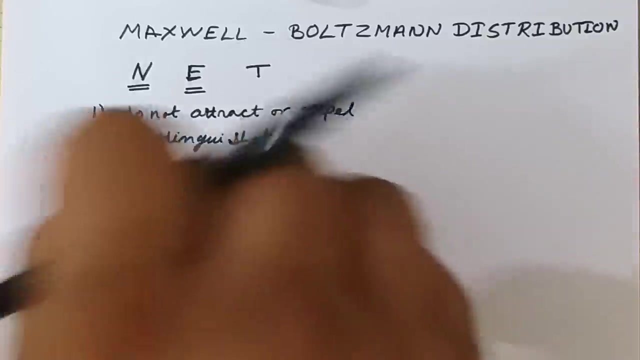 particle, that means any particle can sit anywhere or any particle. we can take any particle from any energy level and we can put that in any energy level. suppose, if a particle is in ground state or E0 energy level, then I can put that particle in E5, E10, E15 or any energy level I want, so there. 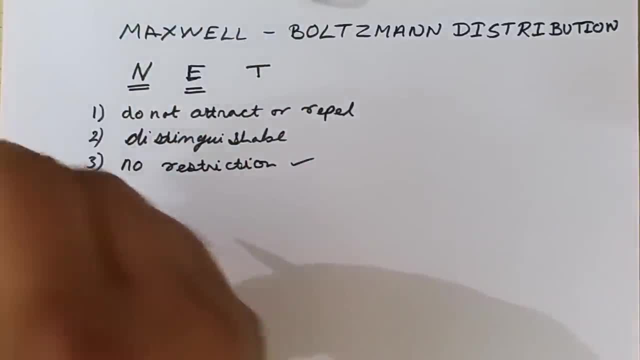 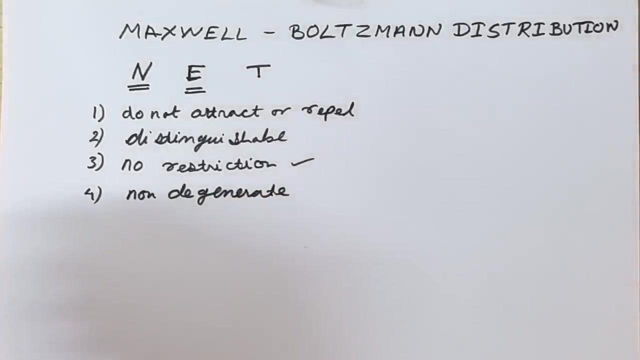 is no restriction on the filling of the energy levels. and the fourth point, or the fourth assumption, is that each energy level is non-degenerate. so each energy level is non-degenerate. so non-degenerate it means that all the energy levels are different. okay, that means. 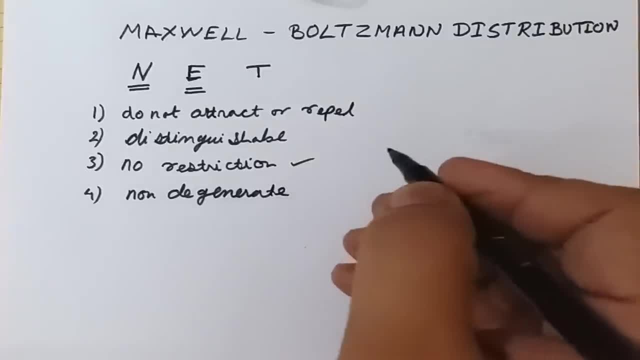 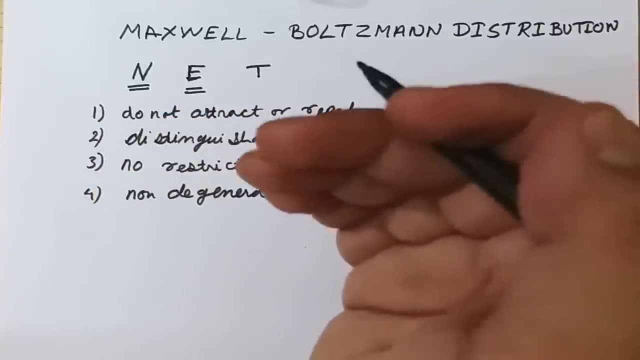 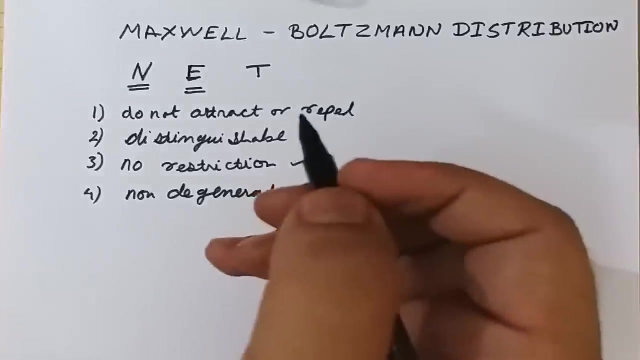 the they are non-degenerate means. suppose if we say E1, E2, E3, E4, E5, then the energy of each energy level is different, and if the energies of the different energy levels are same, then those energy levels would be referred as degenerate energy level. so as we are saying that all the energy 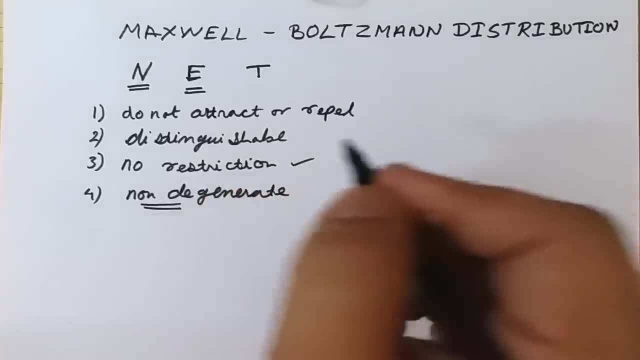 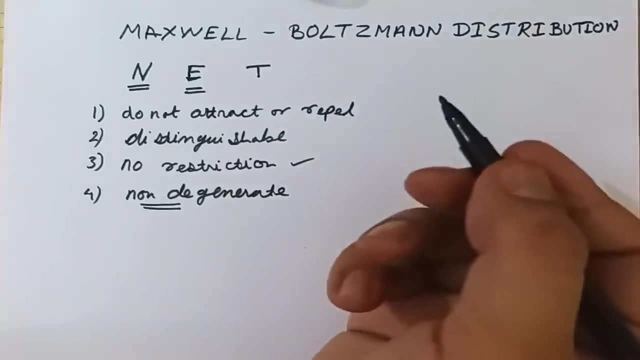 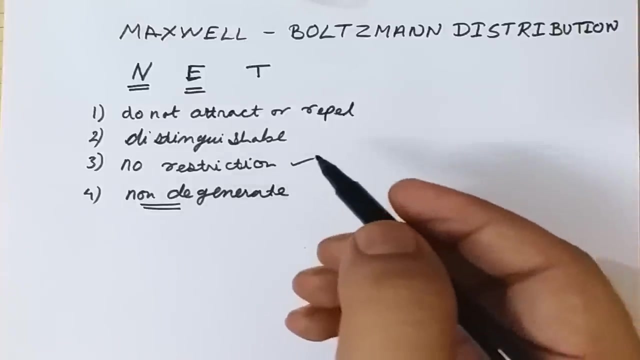 levels are degenerate, so the energy associated with energy level E1 will be different from the ones associated with the energy level E2, E3, E4 and so on. so now, uh suppose, so these are the four assumptions uh, which should be kept in mind before starting the Maxwell Boltzmann distribution law, and 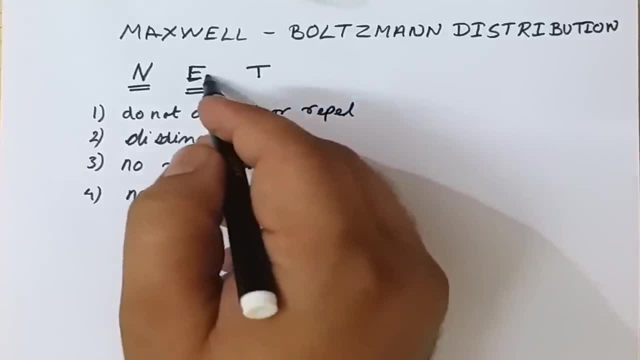 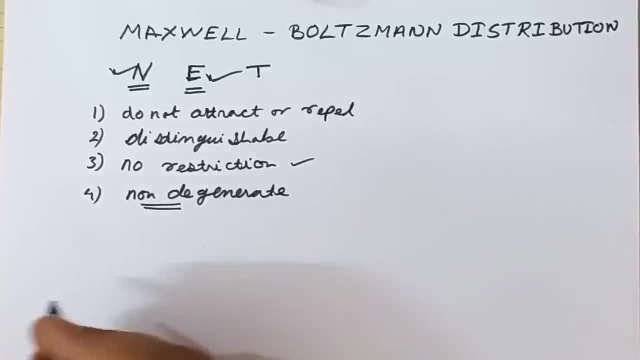 now suppose, if we consider that we are considering that the total amount of the energy is E and we have total number of n number of particles, so if we consider that the total energy levels, they are divided into different energies, like we have E0, E1, E2, E3 and up to E, n, E, n, and we will distribute. 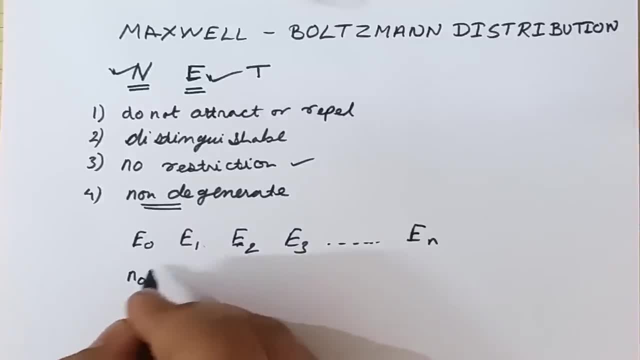 the particles, such that n0 particle will sit in energy level E0, n1 particle will sit in energy level E2, and three and two particles will sit in energy level E2. similarly, and three will sit in n3 particle will sit in energy level E3, and so on, and n particle will sit in energy level n. n okay. 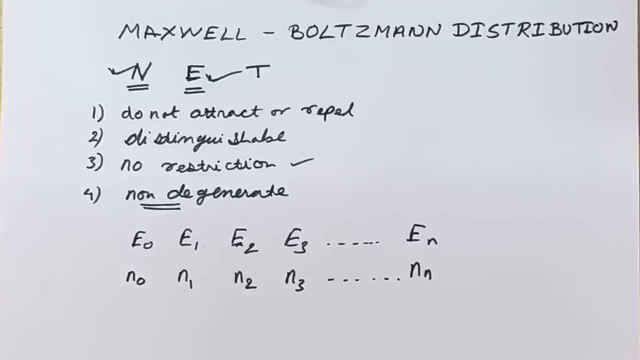 so over here, as we have seen, or irrespective of the distribution, as we know that, irrespective of the distribution, the total number of the particles remains same. or there is uh, according from the first law of thermodynamics, that there is total conservation of energy as well as conservation of 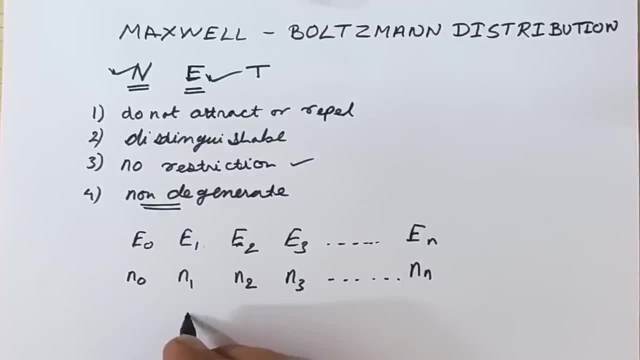 the total number of particles. that is, we can write it as capital, n, or, yeah, we can write it as a total number. that is small: n. that will be equal to summation. i is equal to 1, 2, n, or I can replace it by: for simplicity, for non-confusion, I will replace it by i, so summation i is equal to 1, 2. 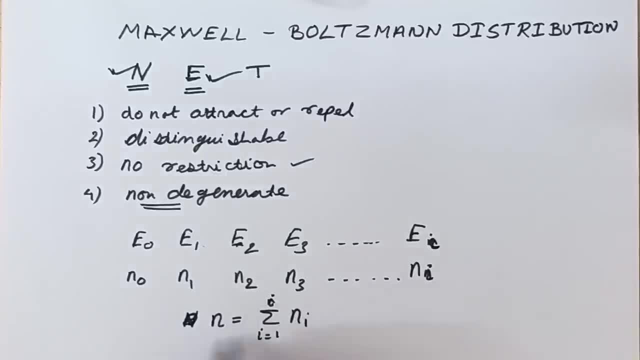 uh, you can say i n, i. the total number is n and similarly the total energy and similarly the total energy E will be equal to summation of. I can write ni ei. so the total energy of energy level E0 will be the total number of particles present in the energy level. total number of particles present in the energy. 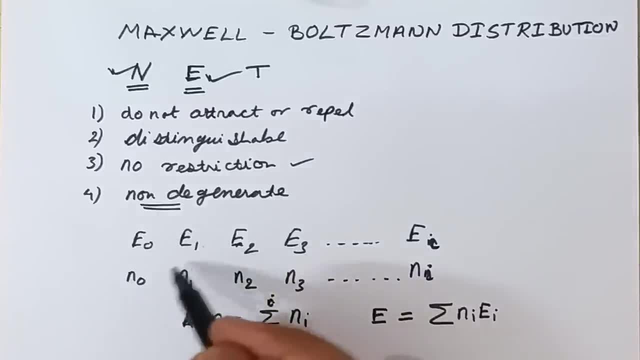 level E0 into the total number of that particle, and similarly for energy level n1, it will be n number of particles present in energy level E1 into total energy of that particular energy level, and hence we can sum it over all the distribution and hence we can get the total energy of the system. now the most probable distribution of this type. 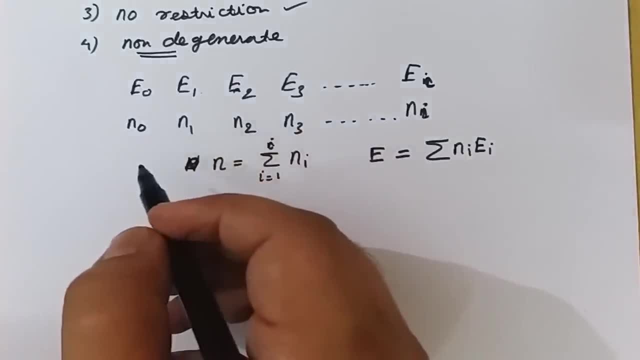 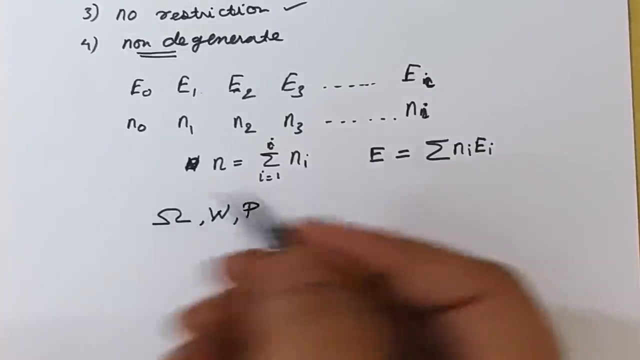 of arrangement. it is given by the thermodynamic probability or most probable distribution. and that most probable distribution. many a times, or in many books, it is written by Omega, or in many books it is written as W, or in many books it is written as P, so we can use any of the notation. uh, I will use Omega or I will use W over here, so we 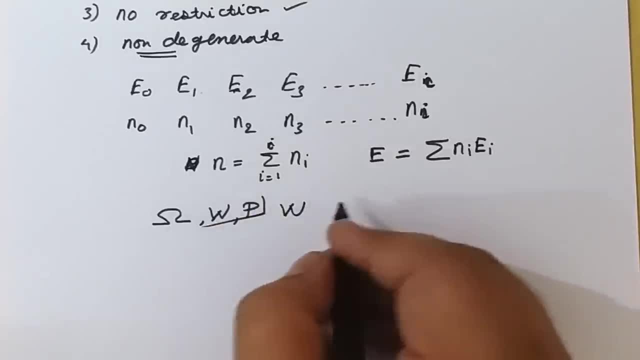 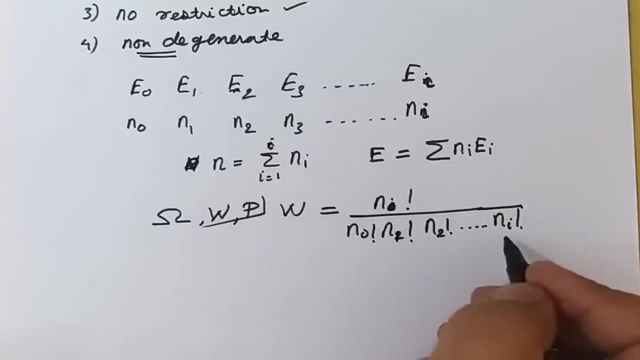 can write W. that is our most probable distribution. that will be equal to. we can write ni factorial upon n zero factorial into 1 factorial, into n 2 factorial. dot, dot dot up to n i factorial. or sorry, total number is n. so total n factorial upon n 0 factorial, n 1 factorial, n 2 factorial up to n i factorial. so this is how we. 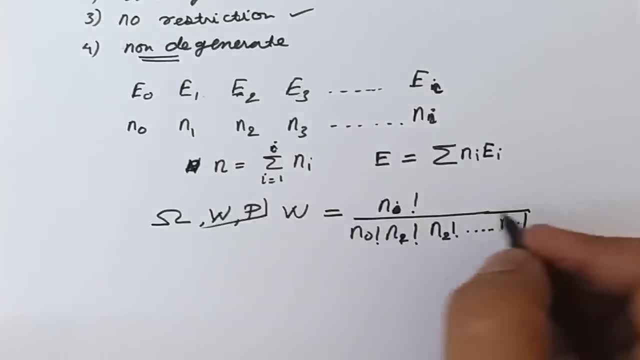 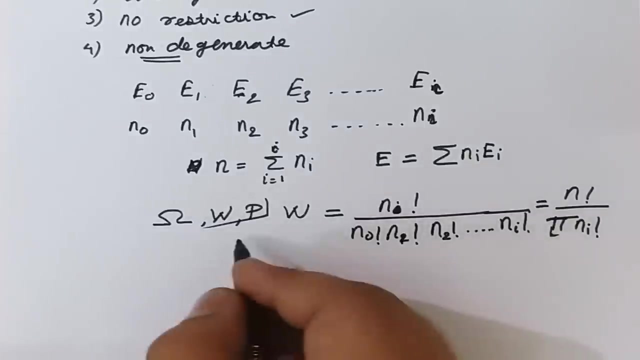 can give the most probable distribution, and I can write this as n? factorial upon capital pi, n i factorial. okay, so, because as we write summation for addition, we for multiplication, we write it by capital pi. now, in order to solve this particular term, what we will do is we can take lon or ln on. 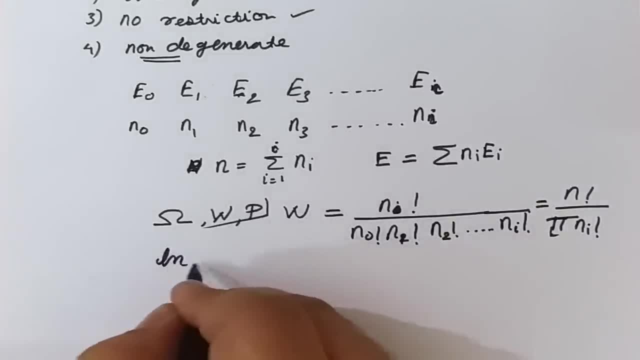 both hand sides. so if we take ln we can have: ln of W will be equal to ln of n factorial. so we know that log of multiplication function is an addition function and when we are taking addition again it will become summation. so we can write summation of ln n i factorial. 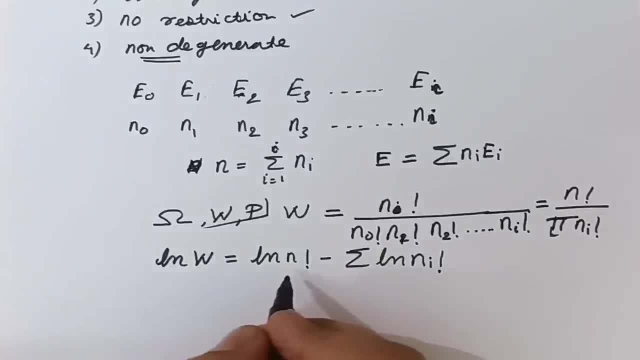 now, as we know that we are having large number of particles. so the solution of such type of term, when we have large number of particles, is given by sterling's approximation formula, and it is. it is given by sterling's approximation and that sterling's approximation is nothing but it is. if we have ln of x factorial, then we can. 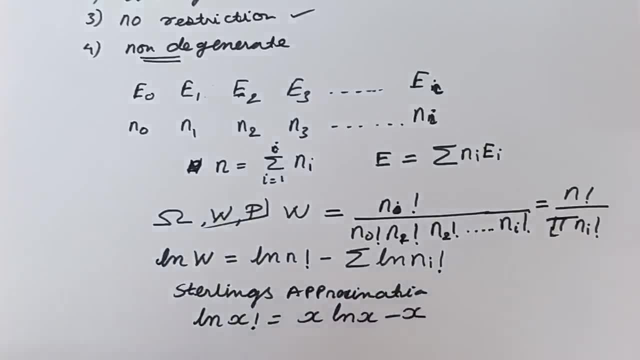 write x, ln, x minus x. so this is sterling's approximation, and this approximation helps to solve the long of a factorial term. and this formula is only applicable for large number of particles or large number of systems or a very large values. so over here, as we are considering that our system contains large number of particles, we can apply sterling's. 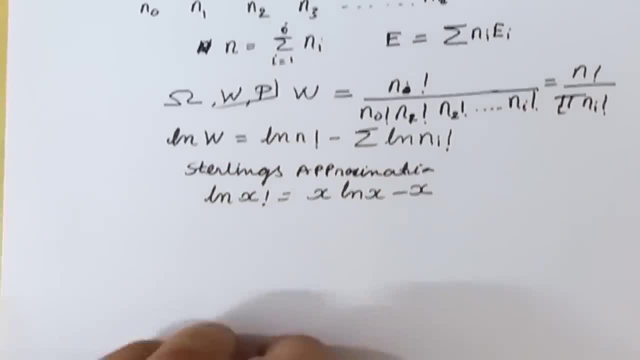 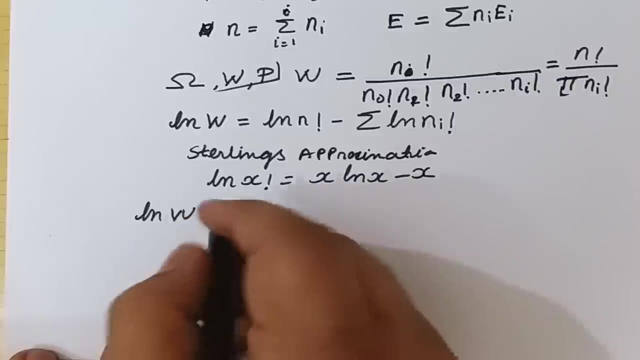 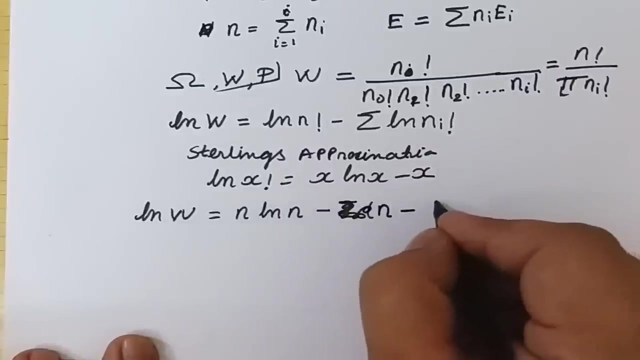 approximation formula to this particular term. so, applying sterling's approximation formula to the term, we will have ln of w will be equal to. we will have n? ln. n minus, n minus, summation n? i, ln, n i minus. that will be plus n? i and as we know that summation of n? i it is. 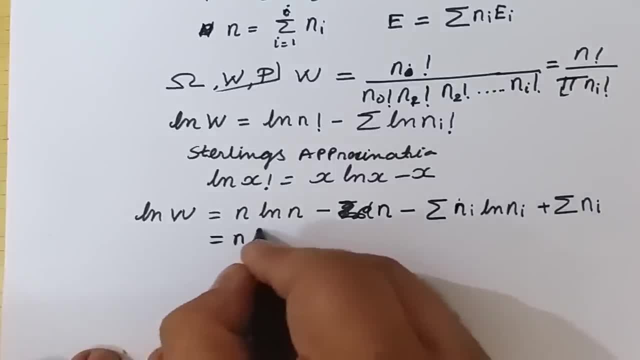 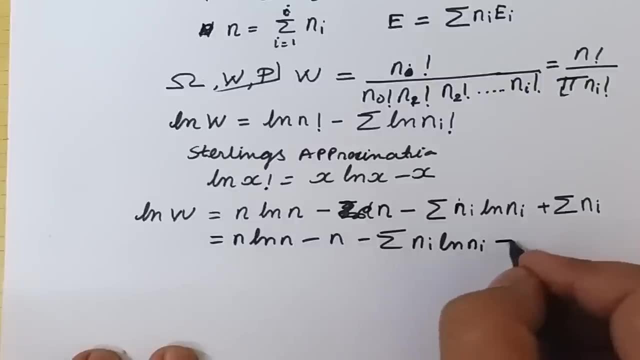 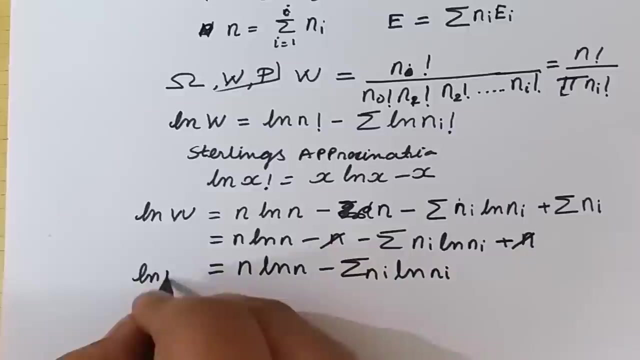 nothing, but it is equal to n. so we can write n ln n minus n minus summation n i ln n i plus n, and both this n will be cancelled out, and hence we will have n ln n minus summation n i ln n i. so we will have ln w or ln omega, or ln p will be equal to. 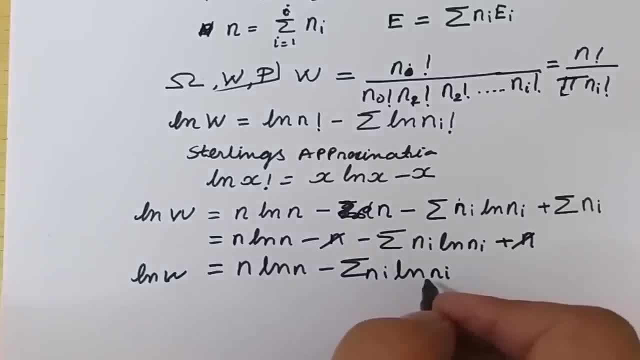 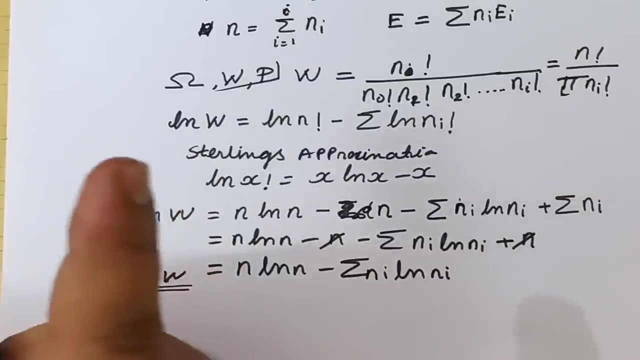 n ln n minus n i ln n i. now, when we are considering that, or in order to find out the most probable distribution, for a most probable distribution, always the system is under equilibrium, okay, and when the system is under equilibrium, there is only a single type of 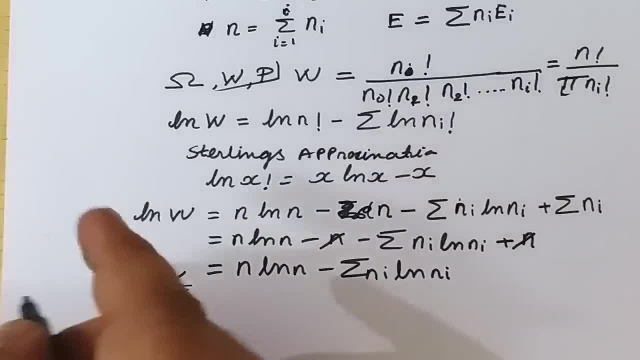 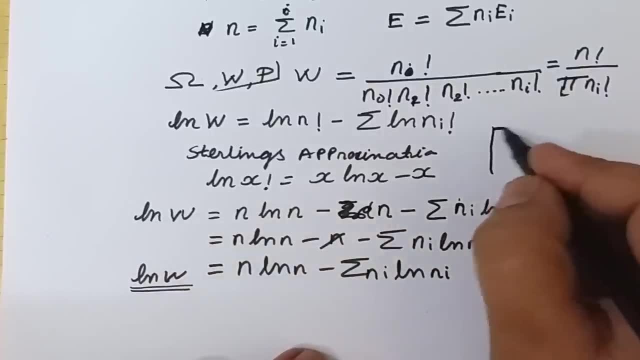 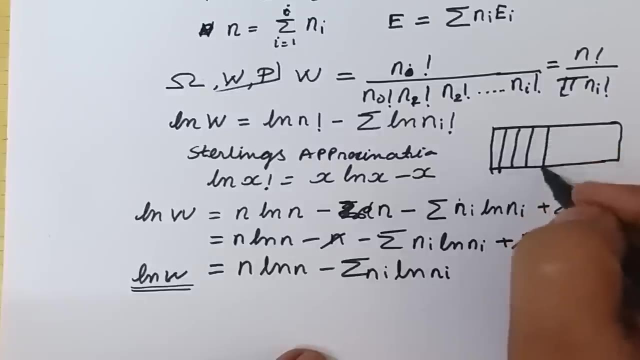 distribution possible or only in a single particular manner we can distribute particle? let me explain by taking one example. that suppose i am having a box. now that box or that box is divided into several number of cells. now in that cells i can individually fill up the gas molecules. okay, and then i have a shutter over here. so now what? 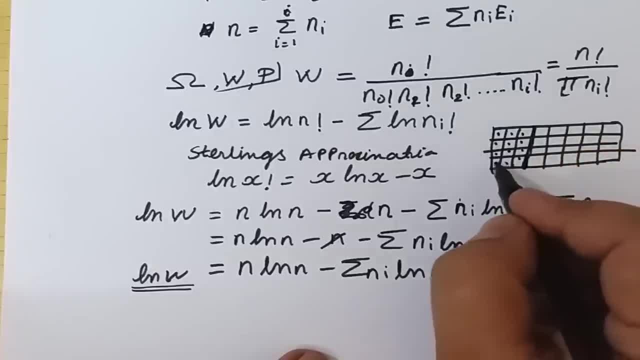 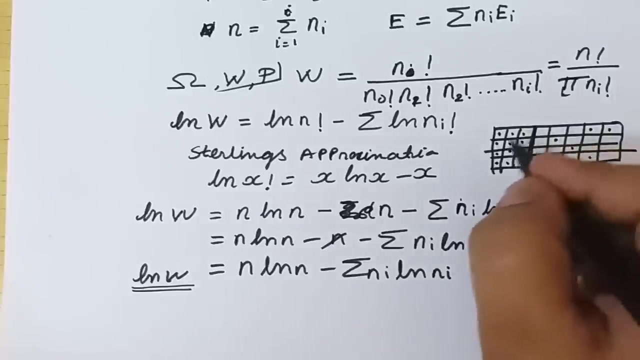 happens when i open this shutter. what will happen? the individual particles will move or they will come out from this and they may occupy several regions in the space or several regions in this particular area, and some will remain in this area. so the particles will stop moving till they have attained the equilibrium. and once they attain the equilibrium, no particle will 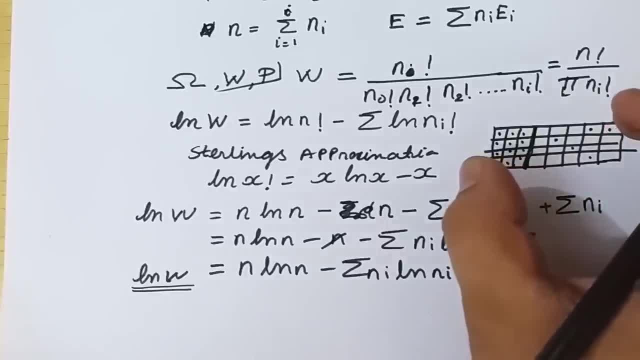 move. okay, and hence that is our most probable distribution. one more example we can take: that suppose in a class, or suppose when a class starts, or before a teacher enters in the class, if the students they enter the class, what will happen? okay, the students will randomly arrange themselves or they will take the respective seat. 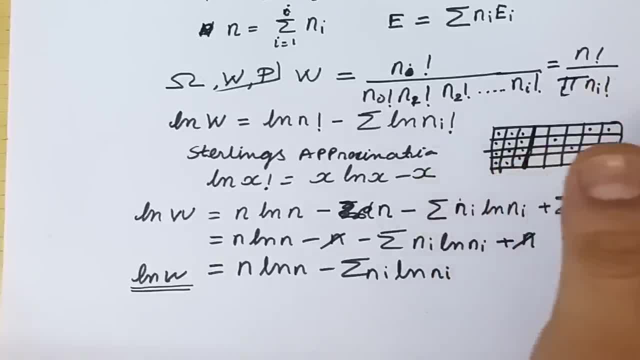 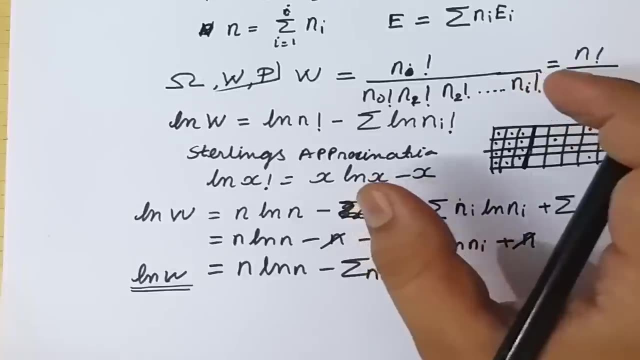 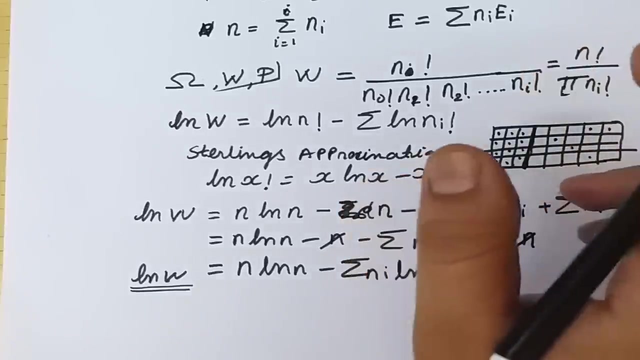 when few of their friends enter. what will happen? they will tend to migrate, but after some times the saturation or after some time the migration of the student stops. that means they are under equilibrium, okay, and hence that particular distribution is the most probable distribution and the most probable distribution is always under equilibrium or the equilibrium position. 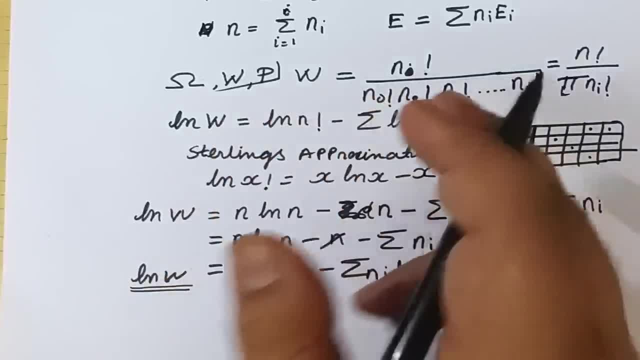 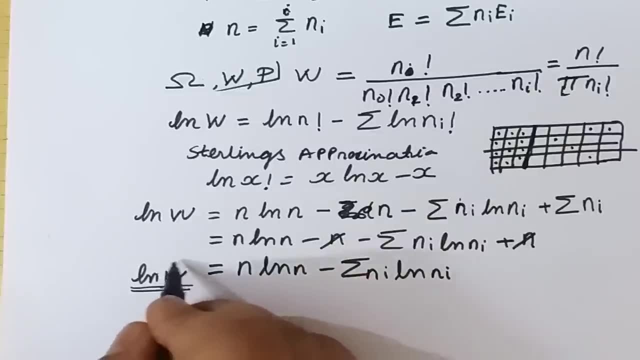 has always the most probable distribution and during the most probable distribution, the value or the value of thermodynamic probability or the value of the most probable distribution is always unity, because there is always single most probable distribution and rest are always less than the most probable distribution. and if we consider this as unity or ln w as a constant term, then the differentiation or 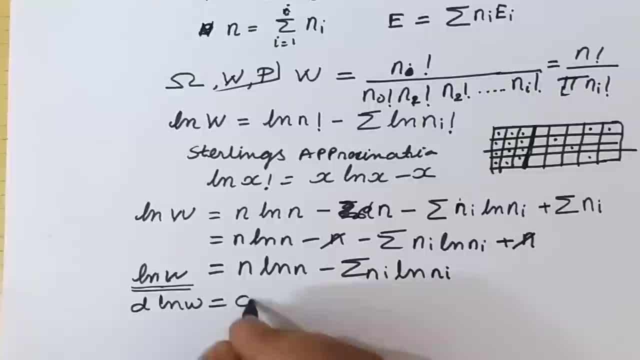 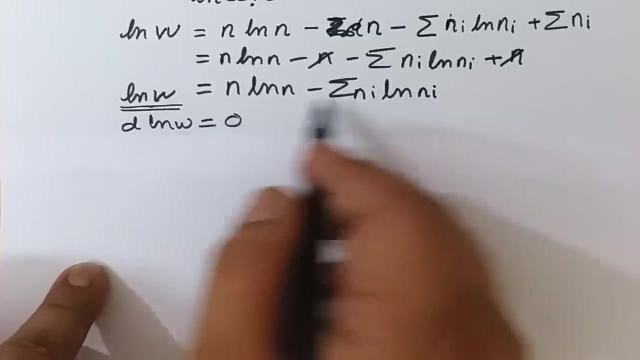 D ln w. we can write it as 0, okay, so what we will do is we will differentiate whole term, or we will differentiate whole term and we will consider that D ln w will be equal to 0 as the most probable for most probable distribution. the value of thermodynamic probability or the value is equal to 0. we will differentiate this particular. 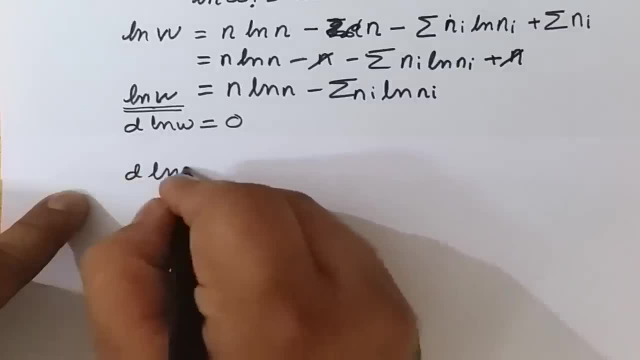 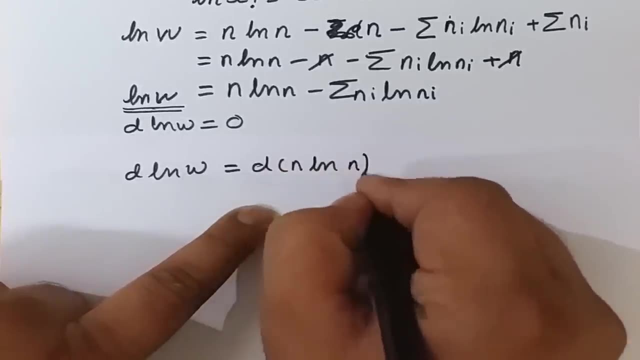 equation. so we will have D ln w. it is equal to differentiation of N ln. N minus differentiation of summation. ni ln N. Mein mod: N N minus 0-dlnWagn, oN2c3, 2 times dLn. 1E2Wn2x2, Rn1e2, Wn2p4x2. 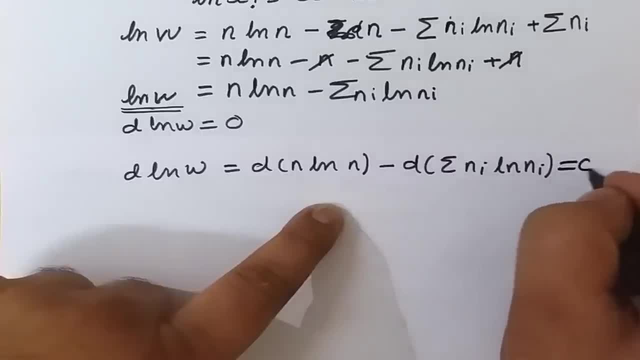 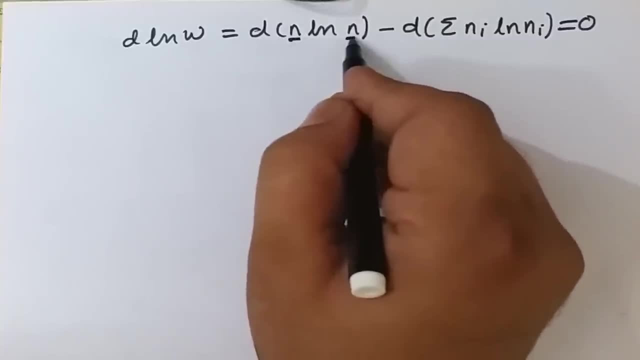 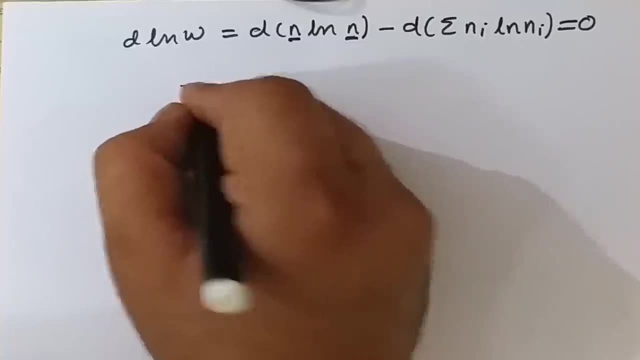 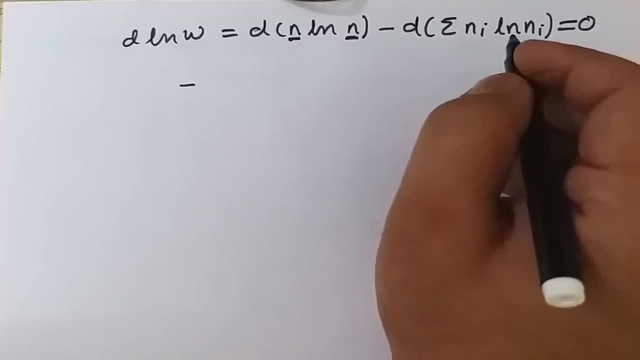 ln ni n. this will be equal to 0. now, over here again, we know that n is a constant term, as well as ln. n is a constant term, so this term will be equal to 0 and hence we will have minus, and we will differentiate this by using the rule of differentiation by parts. okay, and hence we will. 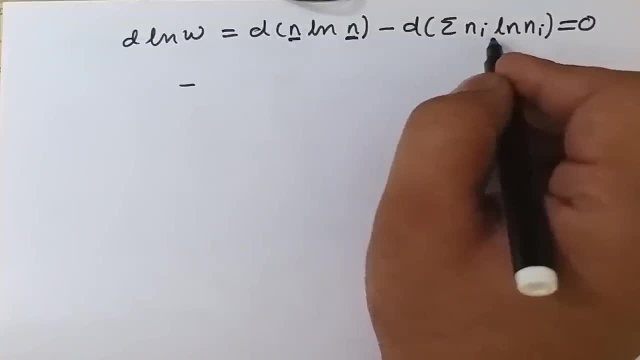 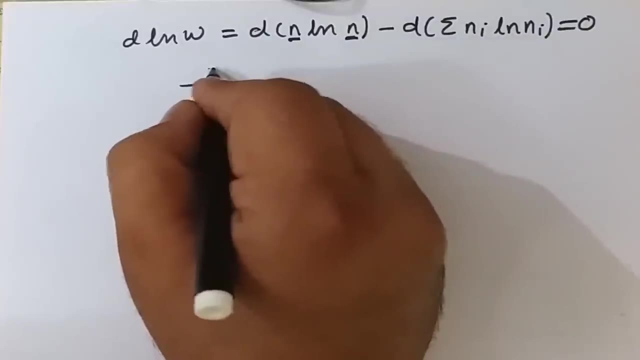 have. we will first differentiate this term, then we will differentiate, or we will first keep one constant, differentiate the other term, and then keep another constant, differentiate the first term, and hence we will have- we can write, i can write summation outside, so minus, and we will have. 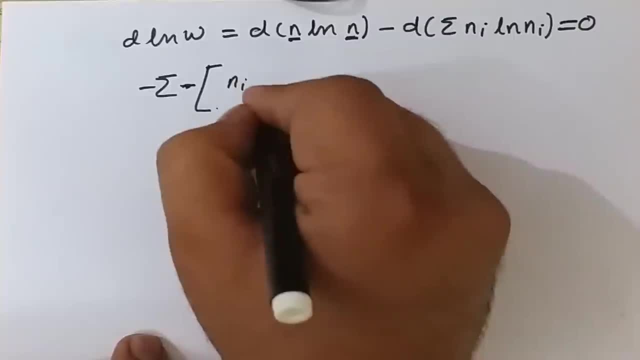 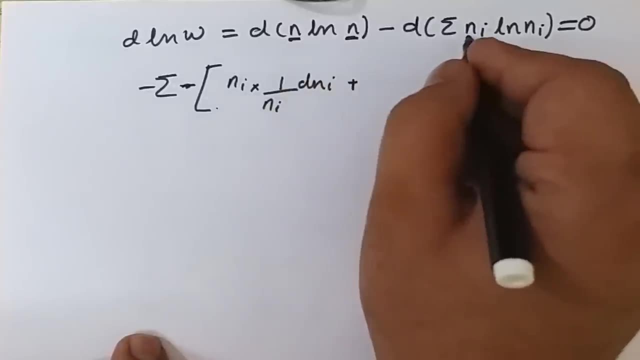 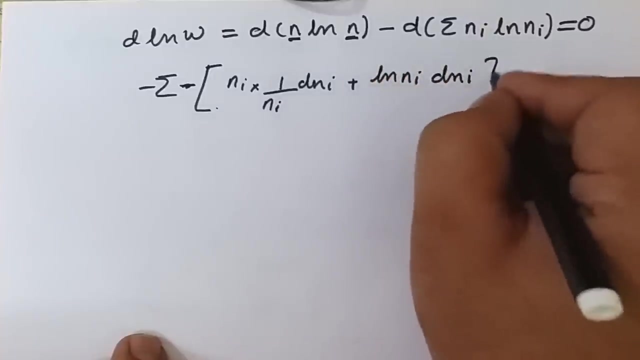 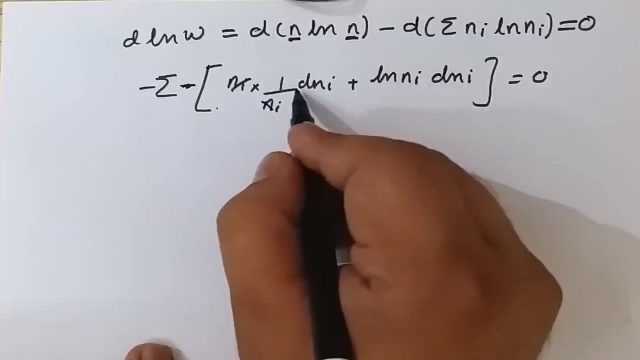 if we keep ni constant, then we will have ni ln of ni is 1 upon ni into dni, plus again, plus again. differentiation of ln ni constant and differentiation of ni will be dni, and that is equal to 0. so both this will be cancelled out and we will have dni plus ln ni dni, and that is equal. 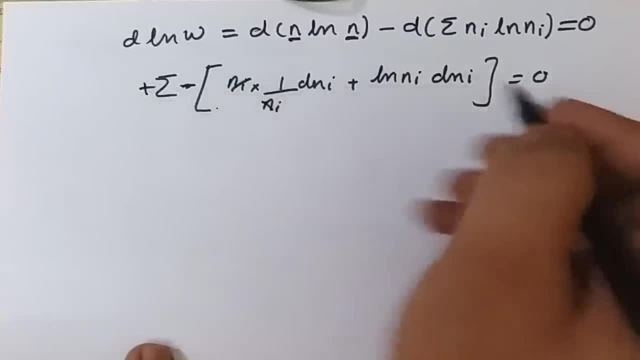 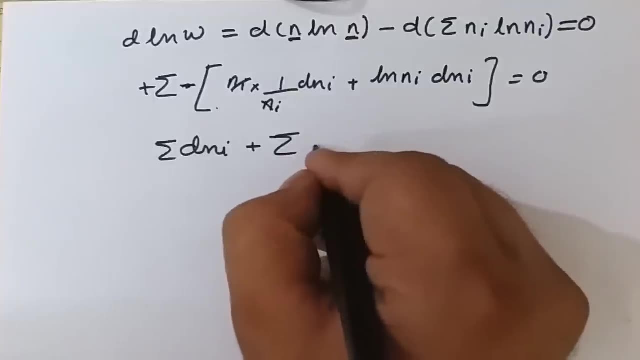 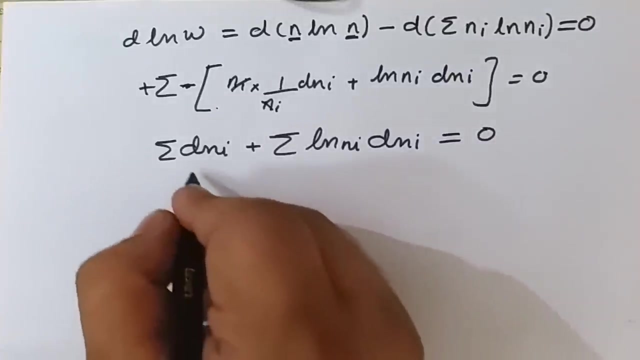 to 0. over here we have minus, so we can multiply both inside by minus and it will become plus. so we will have summation dni plus summation ln ni dni, and that is equal to 0. and again we know that the total number of the particles are constant. and 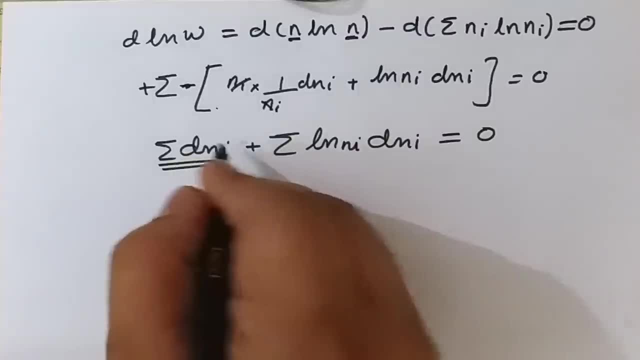 hence summation dni. this will be equal to 0 because the total number of particles are constant and hence, when we differentiate that the is constant and the differentiation will be equal to 0 and hence this term will be equal to 0, so we can write: this term is equal to 0, so we can write summation. 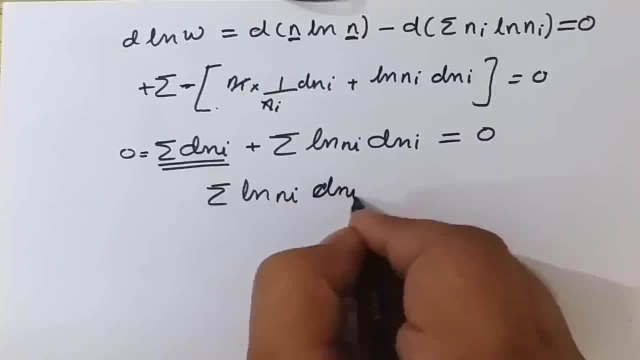 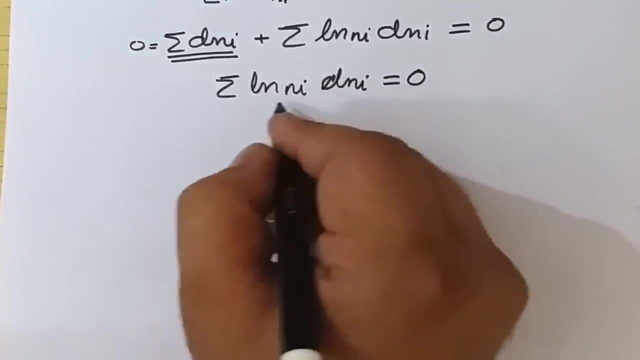 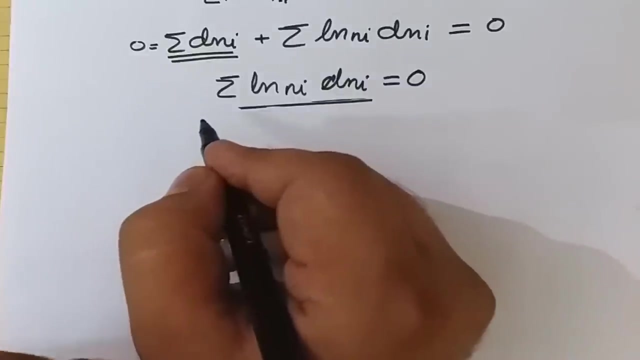 ln ni dni and that is equal to 0. okay, now this term, or now this term. it gives us the most probable distribution now for a system having total amount of, or for a system having total amount of particles, e amount of energy and total n number of particles. okay, and as we have, as we know, that n, we can. 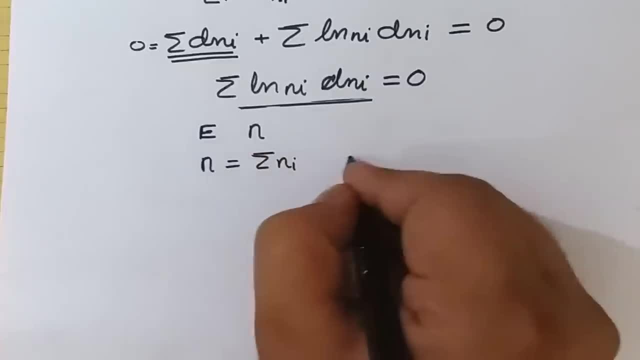 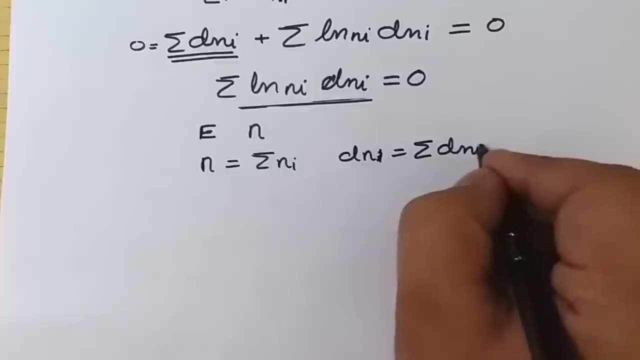 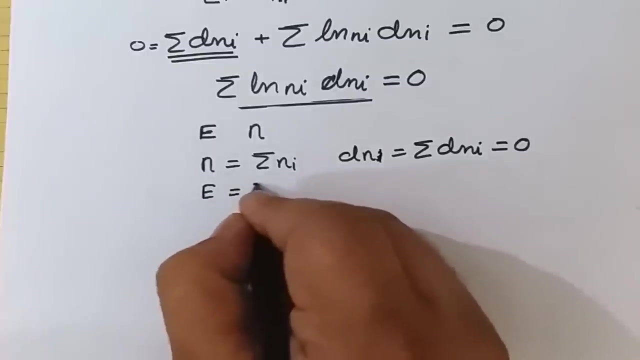 write it as summation n i and if we differentiate this we can have d n i or d n will be equal to summation d n i and that will be equal to zero. and similarly the. we have total energy e and that energy e we can write it as n i into e i. so when we differentiate it we will. 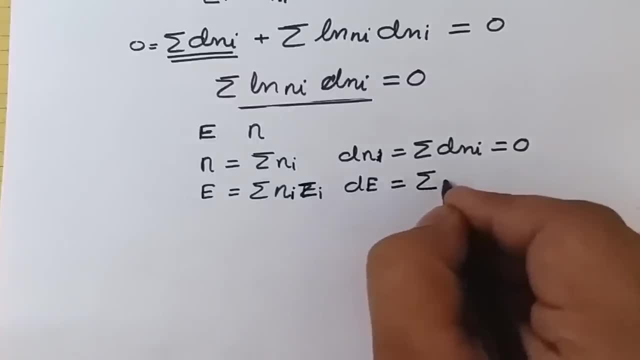 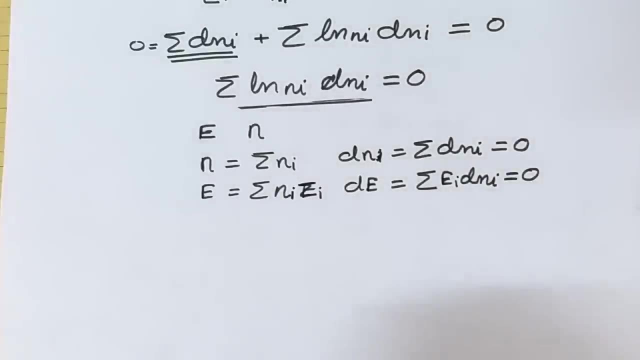 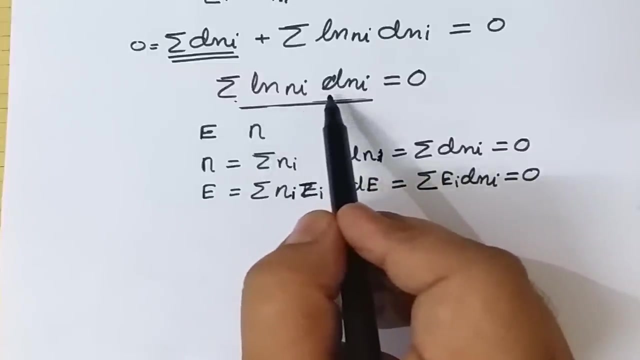 have d, e will be equal to summation of e, i, d, n, i, and that will be also equal to zero, as we know that the total number of particles as well as the total energy of the system it remains constant. okay, so both these will be zero over here. uh, this is our most probable distribution. 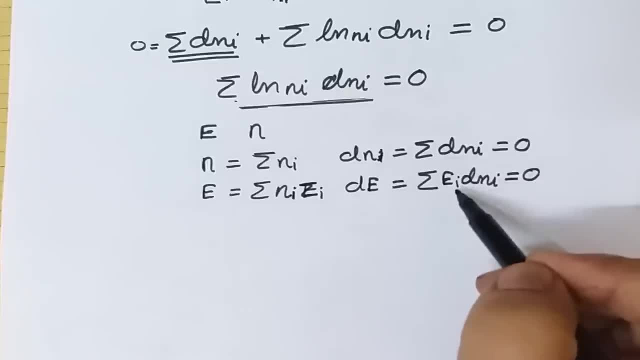 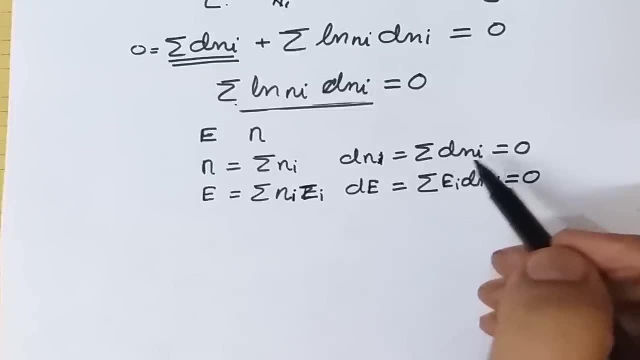 and our most probable distribution is between these two conditions. let me take an example that suppose you are going on a mountain. okay, so mountain has a highest peak and a lowest peak, but you are taking a definite path. so if i tell that, what is the highest point on? 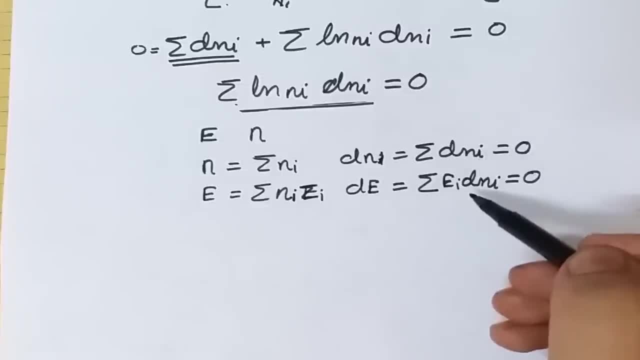 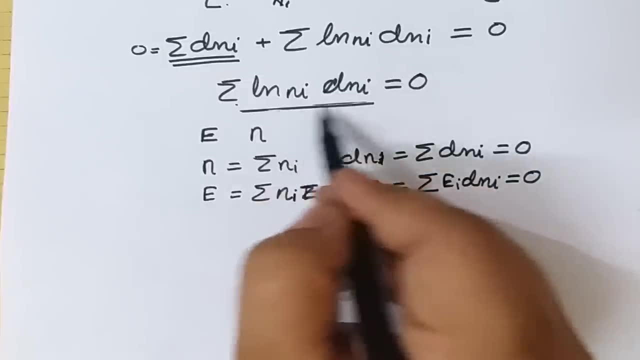 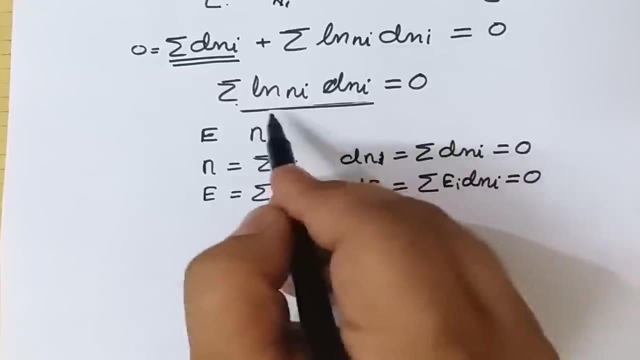 that path. so between and dn, d, n and dn and summation, eidni, so this is our path, and between this path that this is our highest peak. okay, so we are moving along this path and along this path, this is our maximum point, that we are going with, that we are getting, or this is our 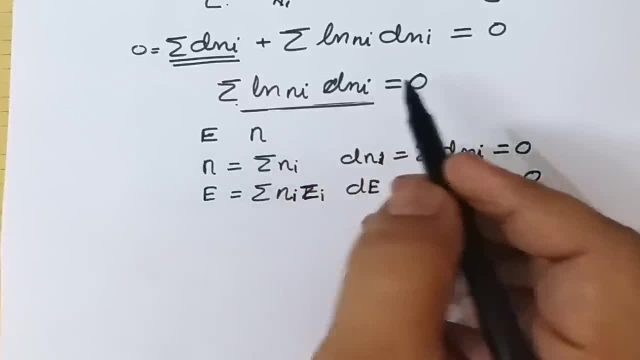 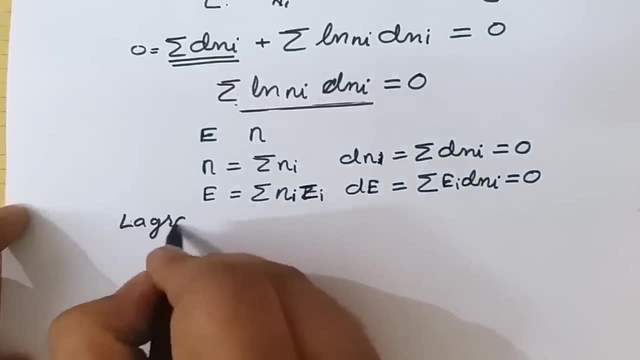 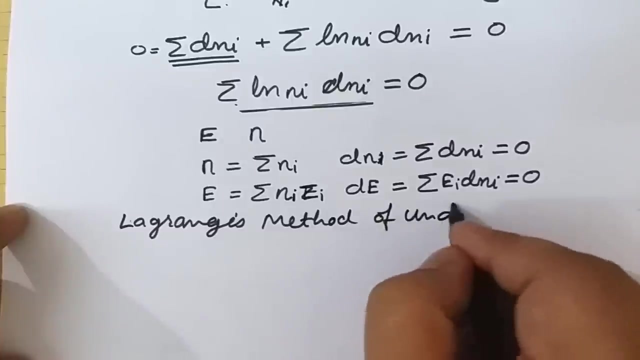 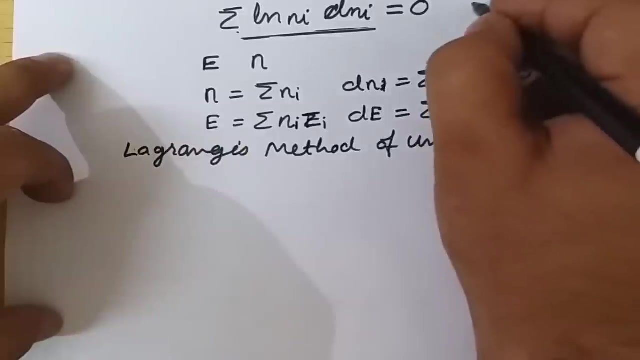 most probable distribution. now there is a method called Lagrange's method of undetermined multiplier. so we will apply Lagrange's method of, we will apply Lagrange's method of undetermined multiplier and what we will do is suppose this is our equation 1, this is our equation 2 and this is our. 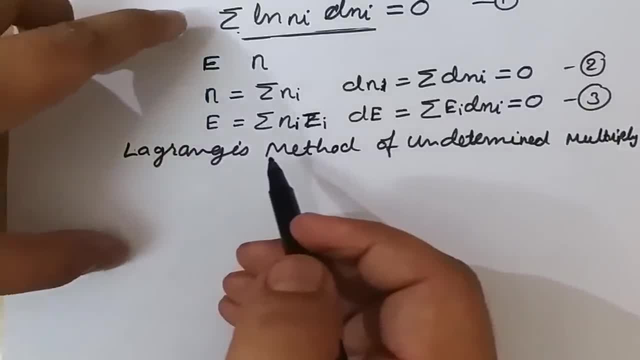 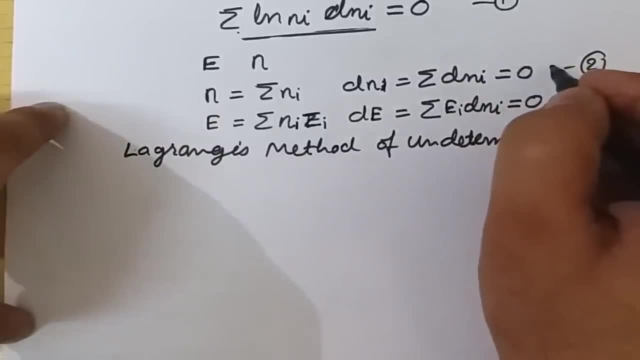 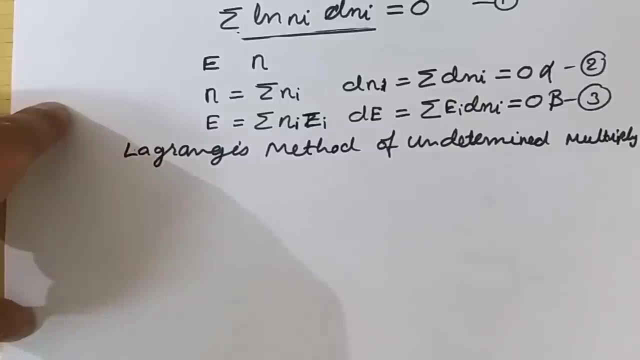 equation 3. what we will do is we will sum up our equation 1, equation 2 and equation 3 in such a way that we will multiply our equation number 2 by alpha and multiply equation number 3 by beta, where alpha and beta they are the constants and they are independent of each other. so we will 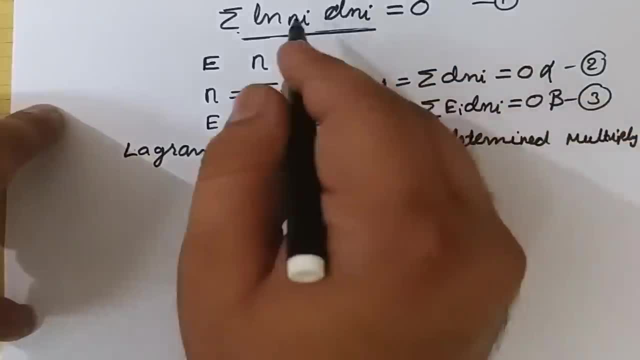 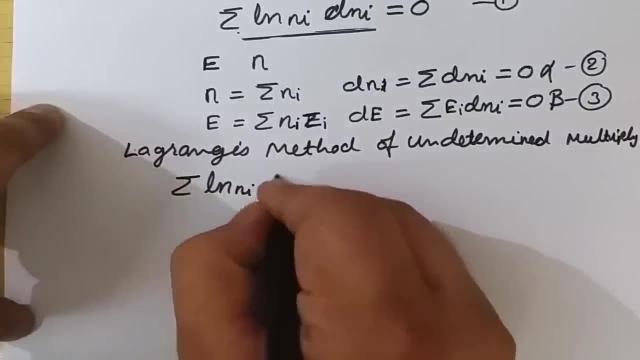 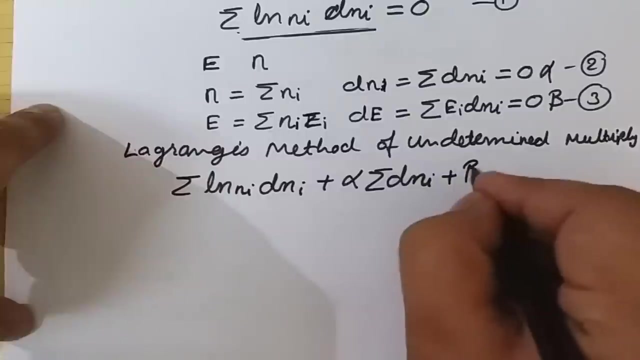 multiply our equation number 2 by alpha, equation number 3 by beta, and then we will add up all the three equations so we will get summation lnnidni plus alpha, summation dni plus beta, summation eidni, and that is equal to zero. we have dni common over here, so we can write. 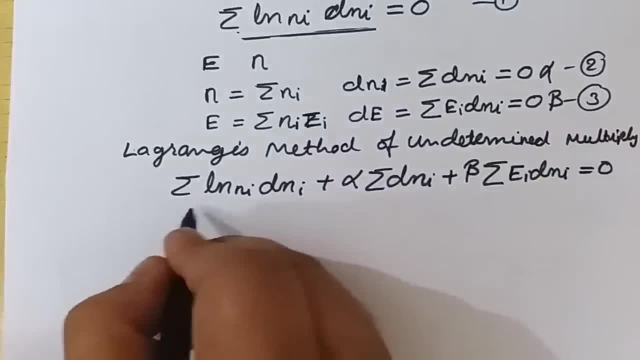 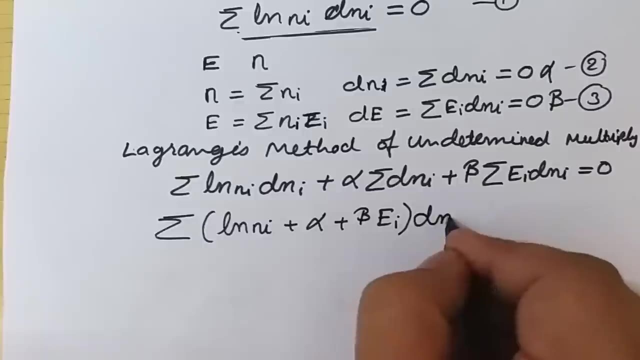 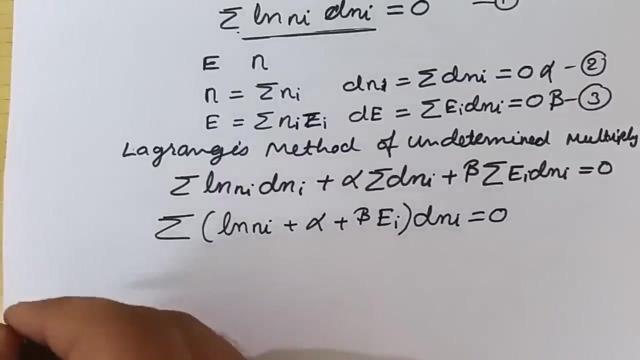 we can take summation as well as dni, so we will have summation ln ni plus alpha, plus beta ei into dni, and that is equal to 0. okay, that is equal to 0, and over here we know that alpha and beta, they are independent of each other. 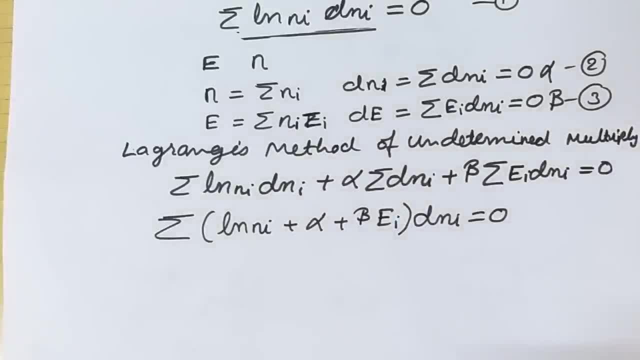 and as we are considering that there are n number of particles in our system, this term, that is dni- it cannot be equal to 0 because, as the we have specific number of particles in the system and for specific number of particles it may, it has certain amount of count and hence this term cannot. 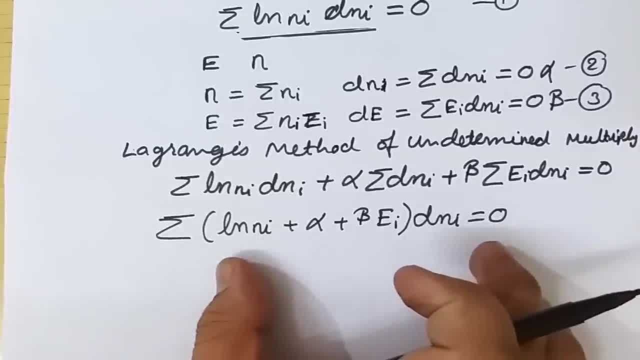 be equal to 0. so, in order to make this particular equation equal to 0, this term must be equal to 0. okay, because this term cannot be equal to 0 as we have certain number of particles in our system. so what we can do is, in order to make this equation equal to 0, this term in the bracket. 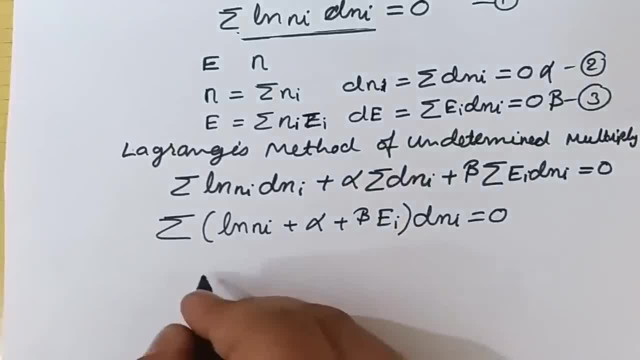 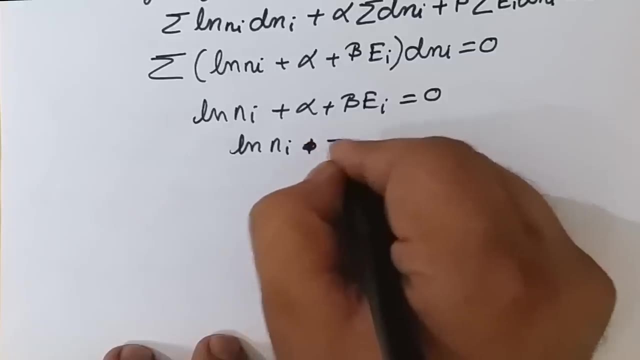 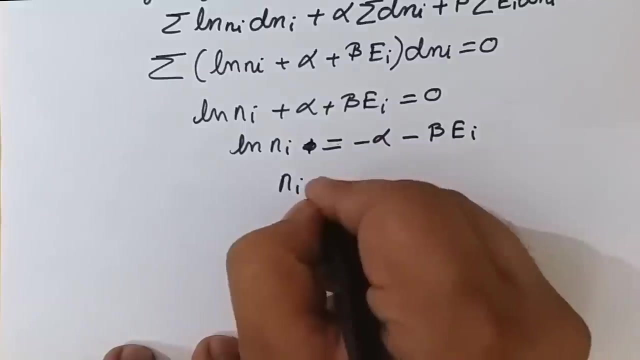 should be equal to 0, and hence we can write ln ni plus alpha, plus beta ei should be equal to 0, so we can rearrange this equation, and hence we can write ln ni. sorry, ln ni is equal to much minus alpha, minus beta ei. so I can write: ni is equal to e raise, to minus alpha, e raise. 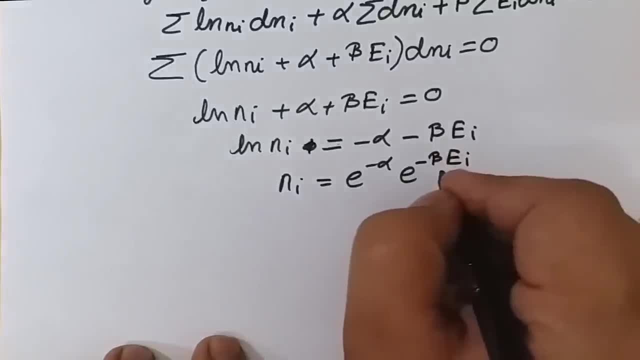 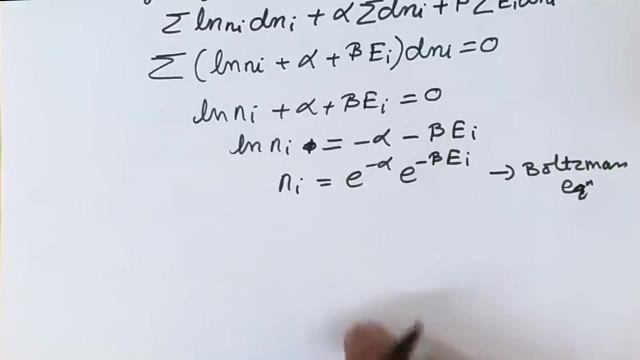 to minus beta ei, okay, and this equation is known as Boltzmann. this equation is known as Boltzmann relation, okay, which gives the distribution of ni number of particles between several energy levels, or it gives us the most probable distribution. we can sum up this equation: 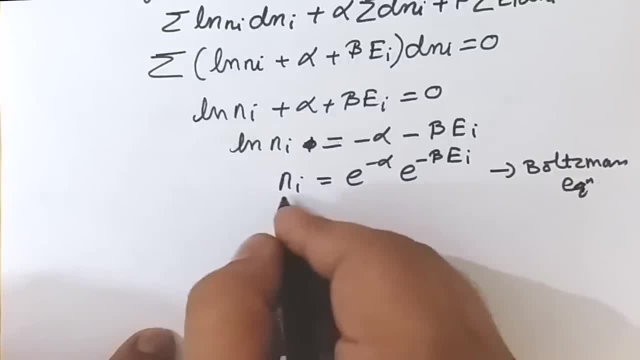 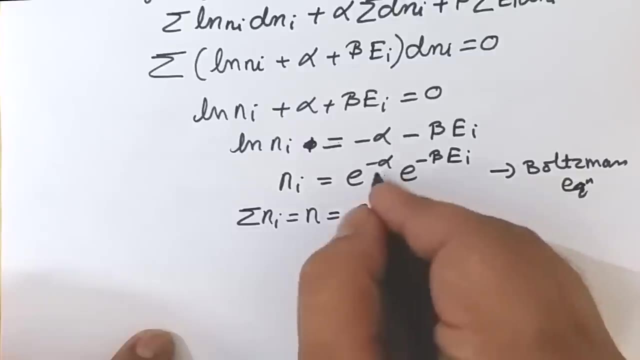 or we can summation, we can sum up this equation for different amount of particles, or we can sum. we can sum this relation and we will get summation ni that. we can write it as n and that is equal to e raise to minus alpha. it is constant. so we can write summation: e raise. 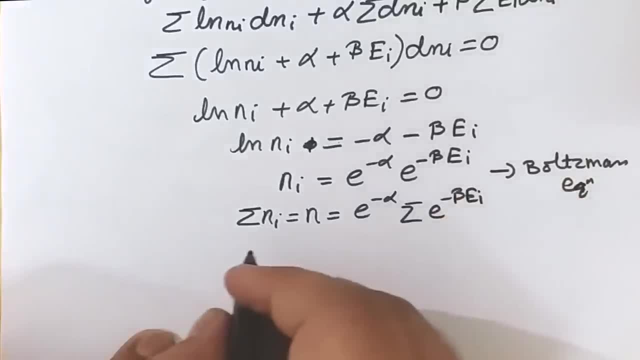 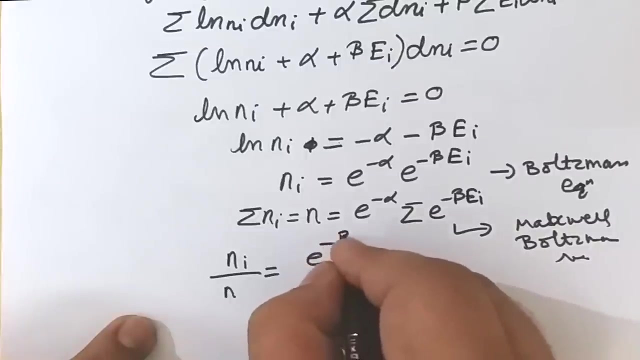 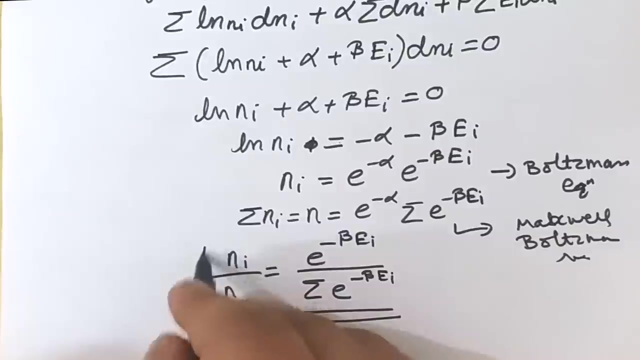 to minus beta ei. okay, so this relation is known as Maxwell-Boltzmann relation. so this equation also gives us the most probable distribution and if we take the ratio of both, this relation then we will have: ni upon n is equal to e raise to minus beta ei. upon summation, e raise to minus beta ei, and this form is the generalized. 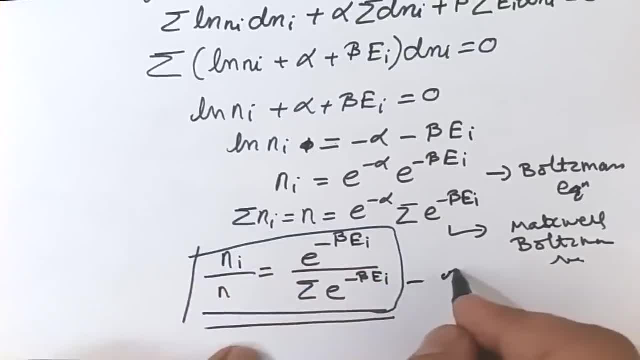 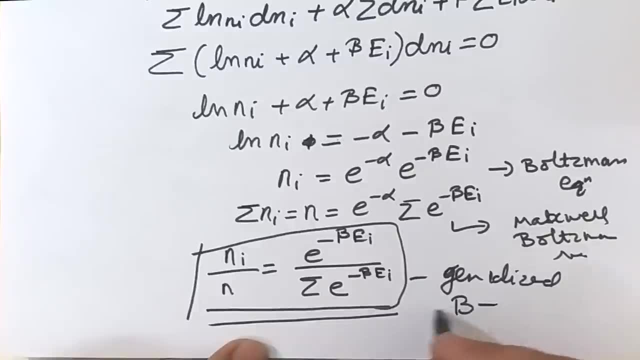 form. so this form is the generalized, this form is the generalized form and this one is not the previous form of Boltzmann and this one is natural form. and if we take the ratio of n, the most probable distribution, we can see that as e higher than. 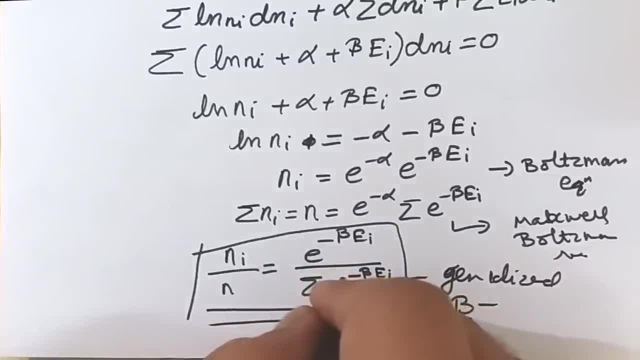 b is the maximum probability of distribution of these particles, or we can write this as t- equal to the maximum boolzman distribution law, and this gives the total population of most probable distribution, or this gives the population of the most probable conflagration of the ensembles, and it is known as canonical distribution. so with the help of this relation we can find out the most probable distribution and the most probable distribution union and the buys and can be taken, this distribution and you will get the founders with you along the way till you have passed, when you test by під. 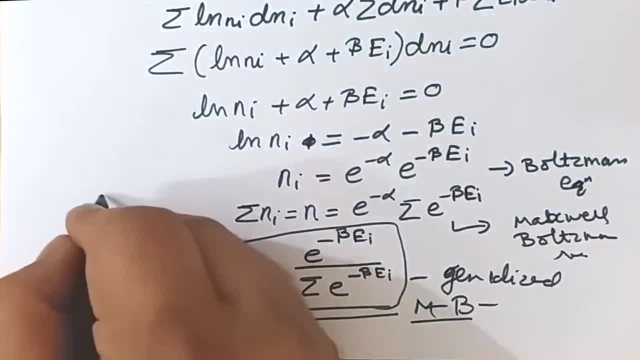 this, you find that the who matched along the second line, whichlingen method of contribution, its equation of division. you can convert it to equal sign of r times y and you take this one as the value of beta. that is, beta is nothing, but it is 1 upon k, t where k is Boltzmann. 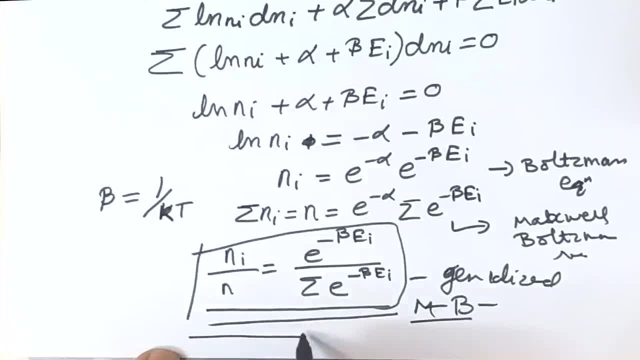 constant Hope the topics are clear. Thank you very much.